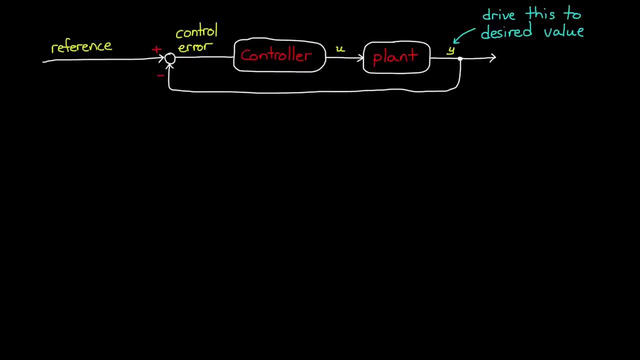 So we're going to create the input signals into the plant with the goal of driving the error to zero. This is the structure of the feedback control system that you would see if you were developing, say, a PID controller, But for pole placement. we're going to approach this problem in a different way. 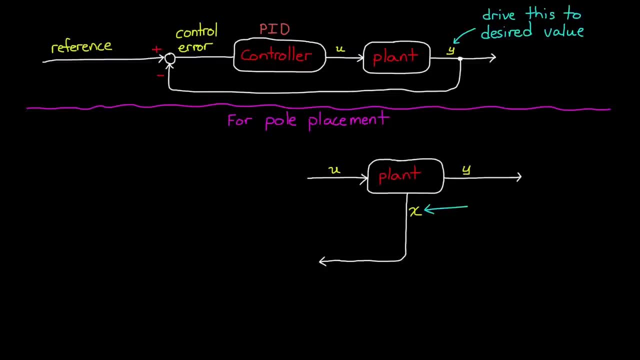 Rather than feedback the output y, we're going to feedback the value of every state variable in our state vector. Now we're going to claim that we know the value of every state, even though it's not necessarily part of the output y, And we'll get to that in a bit, But for 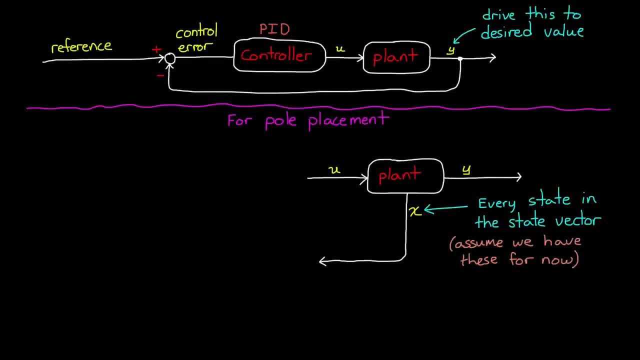 now assume we have access to all of these values. We then take the state vector and multiply it by a matrix that is made up of a bunch of different gain values, And the result is subtracted from a scaled reference signal, And this result is fed directly into our plant. 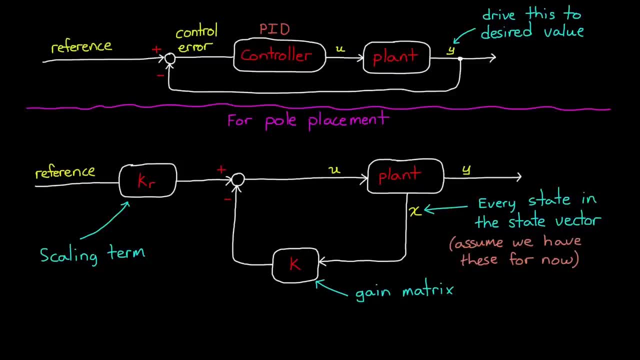 as the input. Now you'll notice that there isn't a block here labeled controller like we have in the top block diagram In this feedback structure. this whole section is the controller And pole placement is a method by which we can calculate the proper gain matrix to guarantee system. 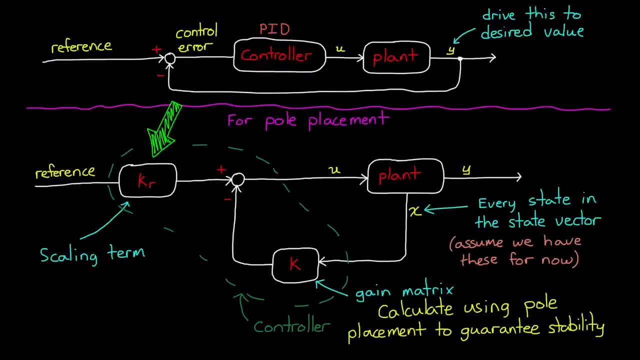 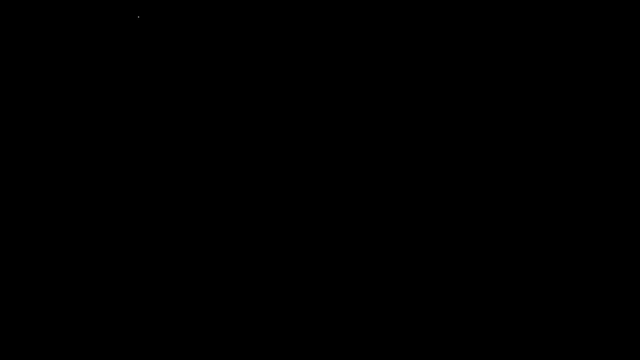 stability, And the scaling term on the reference is used to ensure that steady state error performance is acceptable. I'll cover both of these in this video, But first we need some background information. In the last video we introduced the state equation x dot equals ax plus bu And we 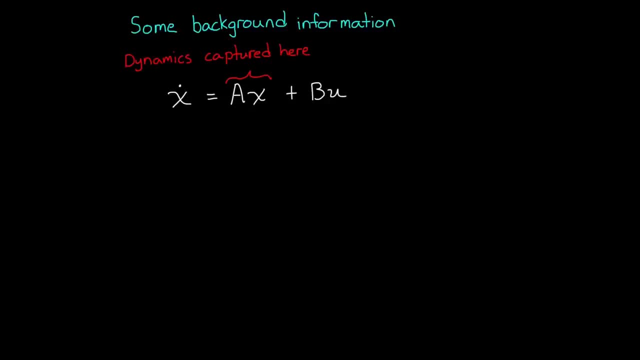 showed that the dynamics of a linear system are captured in this first part, ax. The second part is the energy that is stored in the system. So we can see that the system responds to inputs, but how the energy in the system is stored and moves is captured by the ax term. So you might expect 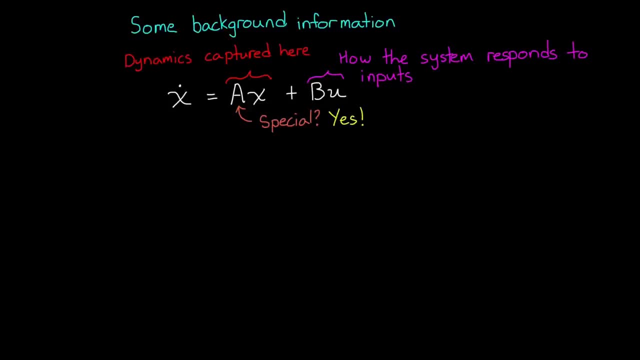 that there's something special about the a matrix when it comes to controller design And there is Any feedback. controller has to modify the a matrix in order to change the dynamics of the system, And this is especially true when it comes to stability. The eigenvalues of the a matrix are the 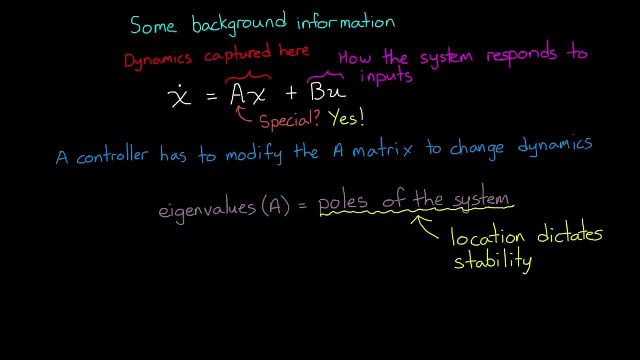 poles of the system And the location of the poles dictate stability of a linear system, And that's the key to pole placement. Generate the required closed loop stability by moving the poles or the eigenvalues of the closed loop, a matrix. Now I want to expand a 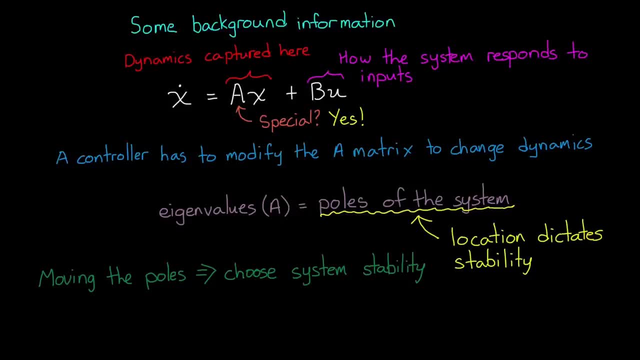 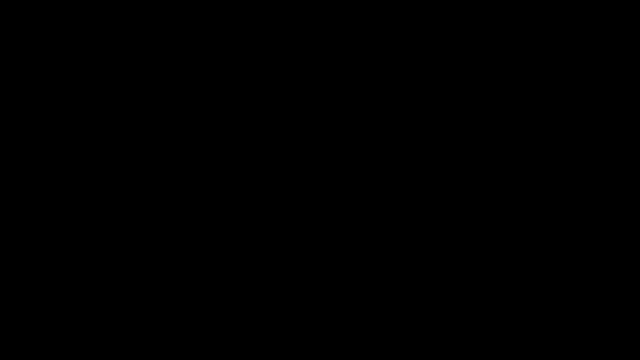 bit more on the relationship between poles and eigenvalues and stability before we go any further, because I think it'll help you understand exactly how pole placement works. For this example, let's just start with an arbitrary system and focus on the dynamics, the a matrix. We can rewrite this in: 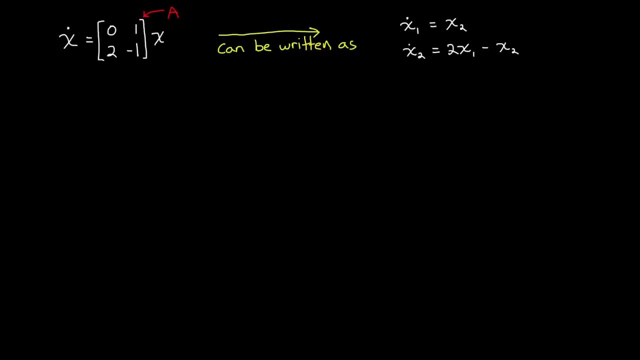 form, so it's a little bit easier to see how the state derivatives relate to the states In general. each state can change as a function of the other states, And that's the case here: x.1 changes based on x2 and x.2 changes based on both x1 and x2.. And this is perfectly acceptable. 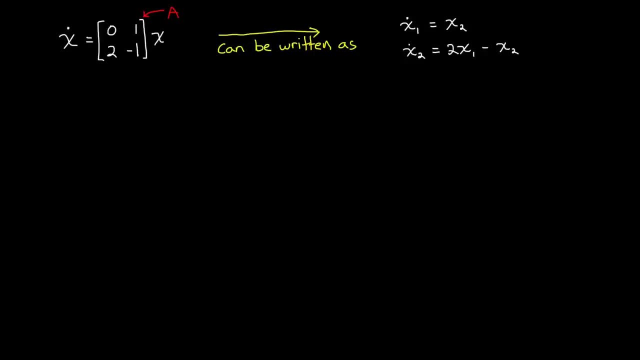 But it makes it a little hard to visualize how eigenvalues are contributing to the overall dynamics. So what we can do is transform the a matrix into one that uses a different set of state variables to describe the system. This transformation is accomplished using a transform. 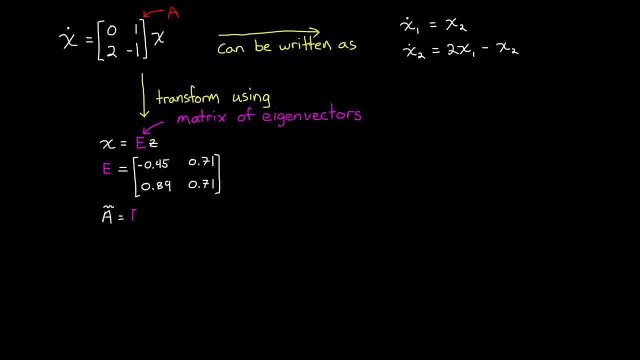 matrix whose columns are the eigenvectors of the a matrix, And what we end up with after the transformation is a modified a matrix consisting of the complex eigenvalues along the diagonal and zeros everywhere else. Now, these two models represent the exact same system. They have the 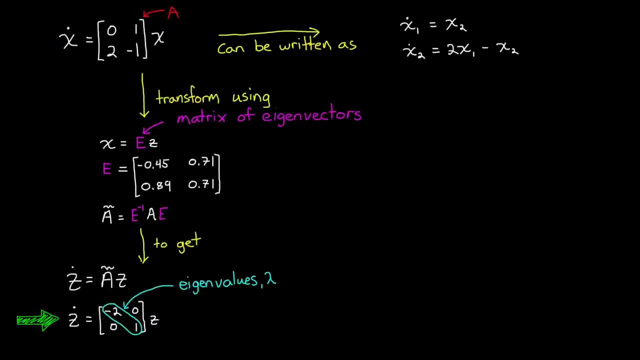 same eigenvalues and the same dynamics. It's just the second one is described using a set of state variables, And this is the first step in the transformation process. So we can see that when we have a set of state variables, we can see that they change independently of each other. 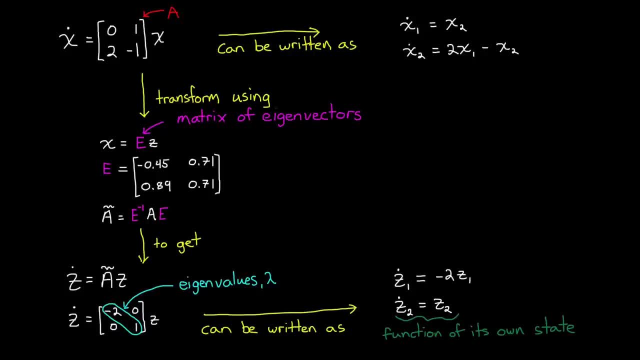 When the a matrix is written in diagonal form, it's easy to see that what we're left with is a set of first order differential equations where the derivative of each state is only affected by that state and nothing else. And here's the cool part: The solution to a differential equation like 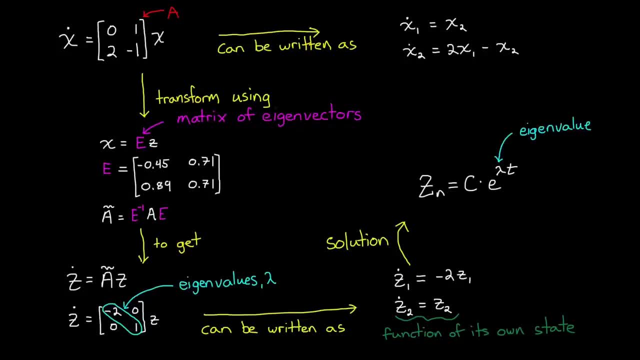 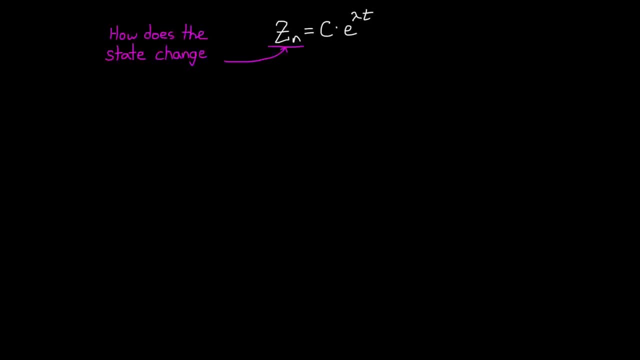 this is in the form. z equals a constant times e to the lambda t, Where lambda is the eigenvalue for z. So let's dive into this equation a little bit more. Zn shows how the state changes over time, given some initial condition, c, Or another way of thinking about this is that if you initialize the 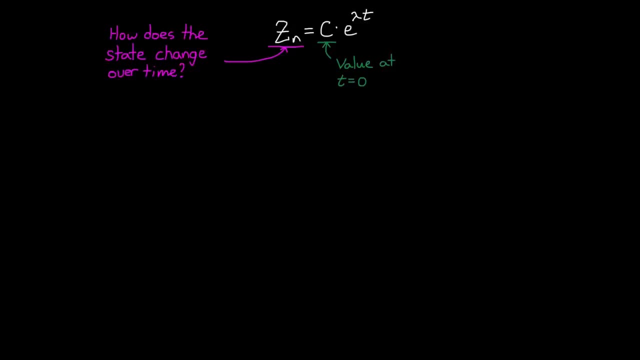 state with some energy or you add energy from an external input. this equation shows how that energy changes And by changing lambda you can affect how the energy is dissipated or, in the case of an unstable system, how the energy grows. So we can visually see how energy changes based on the location of the eigenvalue within the complex plane. 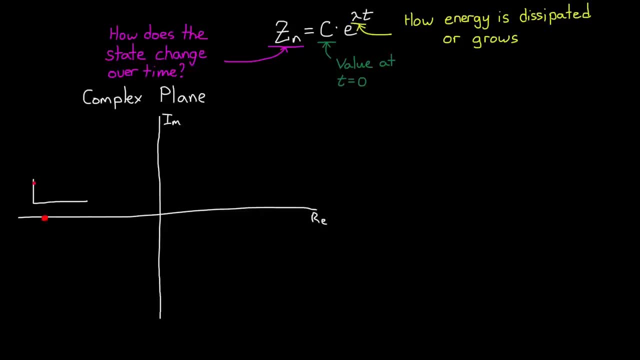 If lambda is a negative real number, then this is a stable eigenvalue, since the solution is e raised to a negative number and any initial energy will dissipate over time. But if it's positive, then it's unstable, because the energy will just grow over time. And if there's a pair, 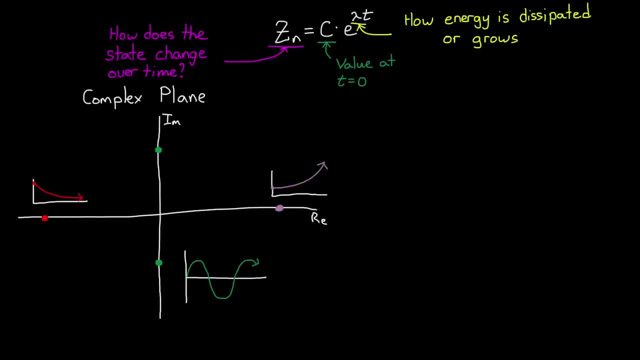 of imaginary eigenvalues, then the energy in this mode will oscillate, since e raised to an imaginary number. So the energy in this mode is just a simple negative. but the energy in this mode is just an example of how the energy in the complex plane does the same thing. So the 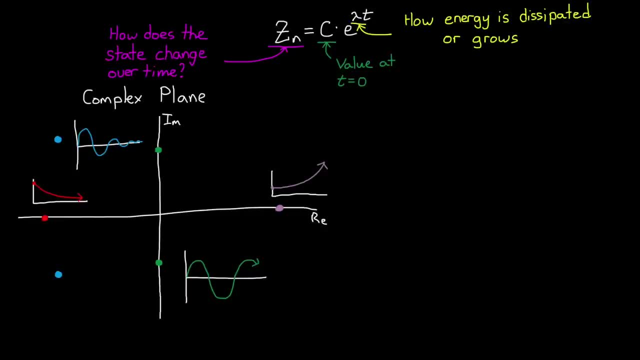 energy in the complex plane is an initial value that produces signs and cosines, And any combination of the two, of real and imaginary numbers, will produce a combination of oscillations and exponential energy dissipation. Now, I know this was all very fast, but hopefully it made enough. 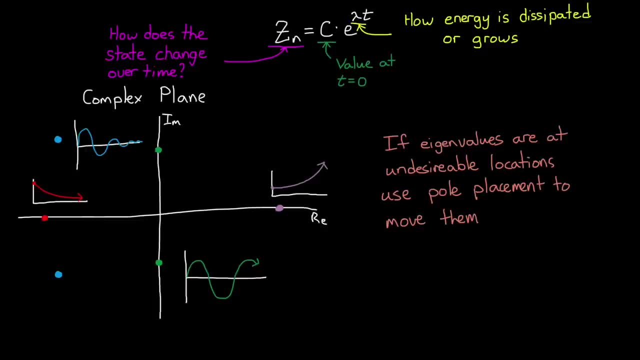 sense that now we can state the problem we're trying to solve. If our plant has eigenvalues that are at undesirable locations in the complex plane, then we can use pole placement to move them somewhere else- undesirable, since they'd be unstable, but undesirable could also mean there's oscillations. 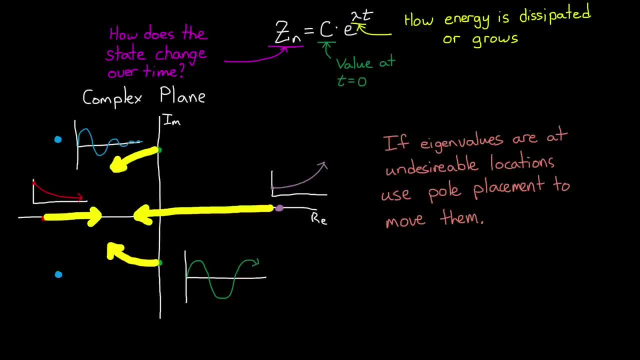 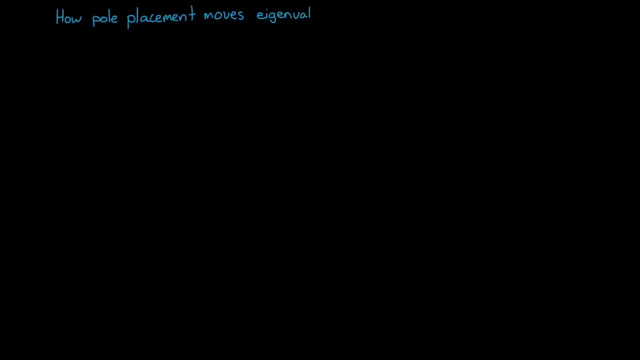 you want to get rid of, or maybe just speed up or slow down the dissipation of energy in a particular mode. With that behind us, we can now get into how pole placement moves the eigenvalues. Remember the structure of the controller that we drew at the beginning? Well, this results in an input u. 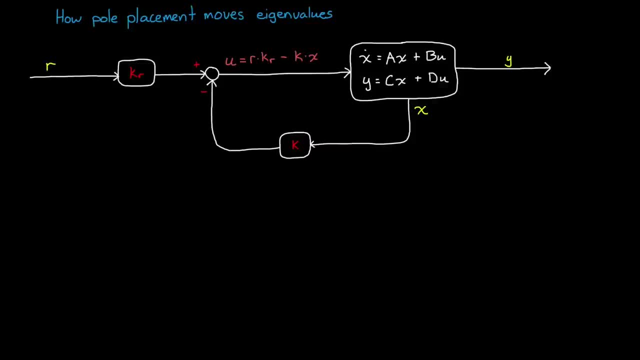 equals rkr minus k times x, where rkr is the scaled reference, which again we'll get to in a bit, and kx is the state vector that we're feeding back, multiplied by the gain matrix. Now here's where the magic happens: If we plug this control input into our state equation, we're closing the. 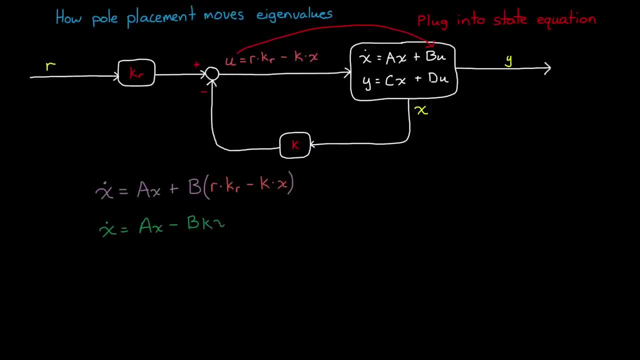 loop and we get the following state equation. Notice that a and minus bk both act on the state vector, so we can combine them to get a modified state. A matrix- This is the closed loop- a matrix, and we have the ability to move the eigenvalues by. 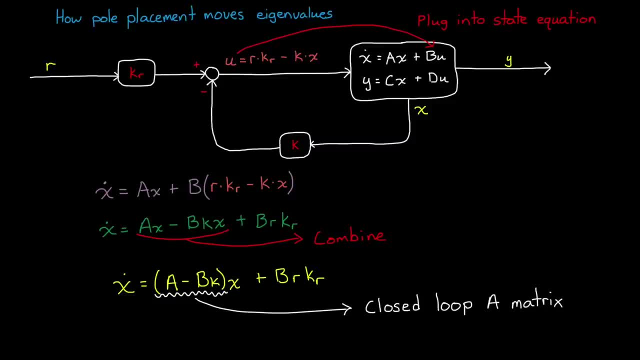 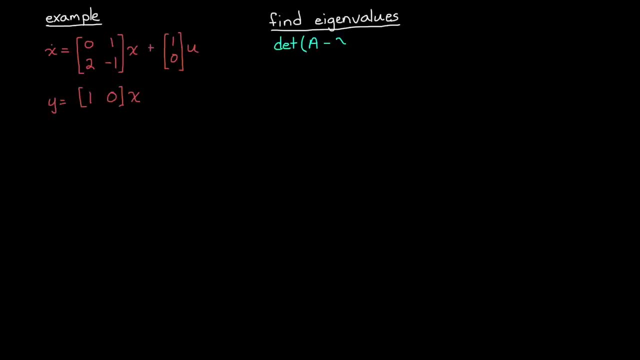 choosing an appropriate k, and this is easy to do by hand for simple systems. Let's try an example with a second order system with a single input. We can find the eigenvalues by setting the determinant of a minus lambda i to zero and then solve for lambda and they're at minus two and 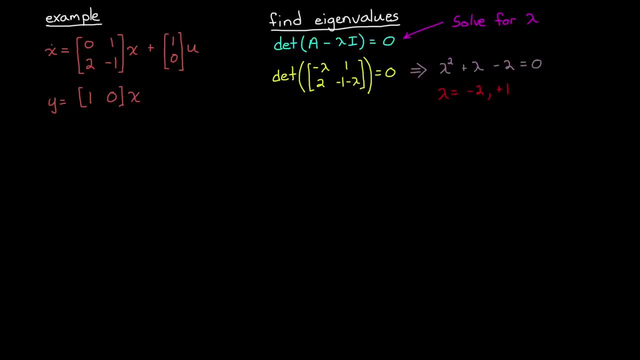 plus one, One of the modes will blow up to infinity because of the presence of the positive realtor. If we plug this into a closed loop, a matrix, we can find the eigenvalues of a minus bk, and so the system as a whole is unstable. Let's use pole placement to design a feedback. 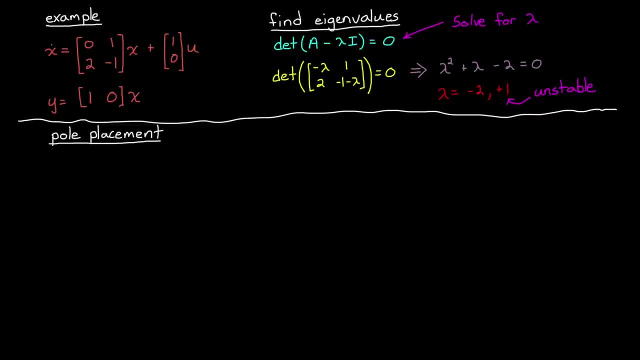 controller that will stabilize this system by moving the unstable pole to the left half plane. Our closed loop: a matrix is a minus bk and the gain matrix k is a one by two. since there's one output in two states, This results in minus k one, one, minus k two, two and minus one. 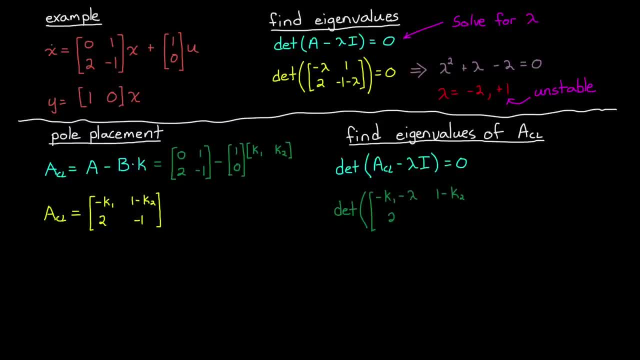 and we can solve for the eigenvalues of acl like we did before. Now let's say that we want our closed loop poles at minus one and minus two. In this way, the characteristic equation needs to be lambda squared plus three times lambda plus two equals zero. 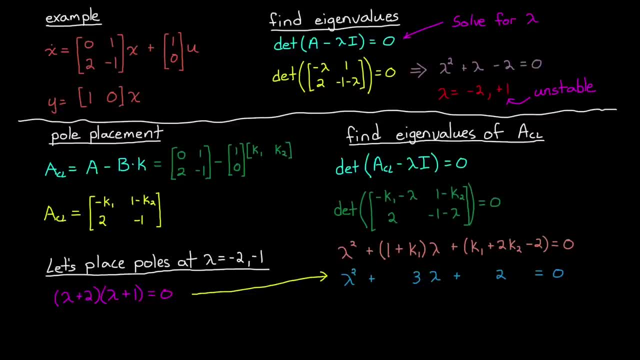 And at this point it's straightforward to find the appropriate k one and k two that make these two equations equal. We just set the coefficients equal to each other and solve and we get k one equals two and k two equals one, And that's it. If we place these two gains in the state feedback. 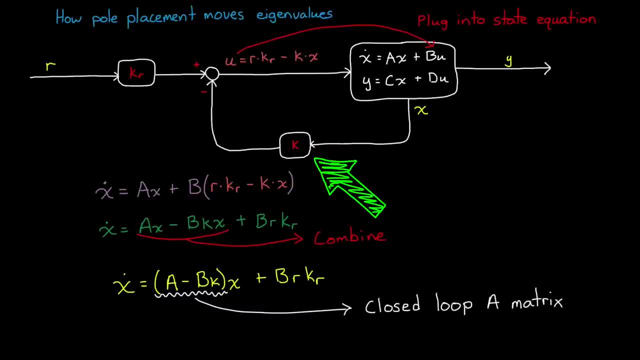 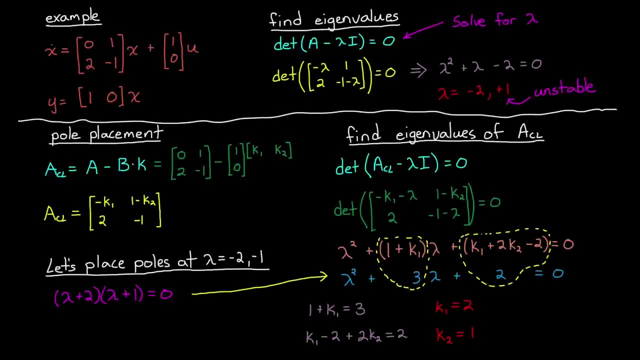 path of this system. it will be stabilized with eigenvalues at minus one and minus two. Walking through an example by hand, I think, gives you a good understanding of pole placement and how it works. However, the math involved starts to become overwhelming for systems that have more. 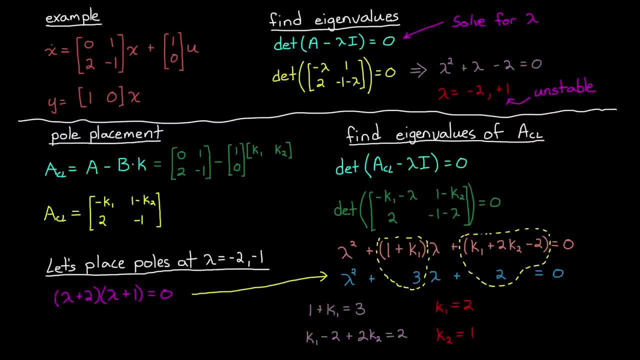 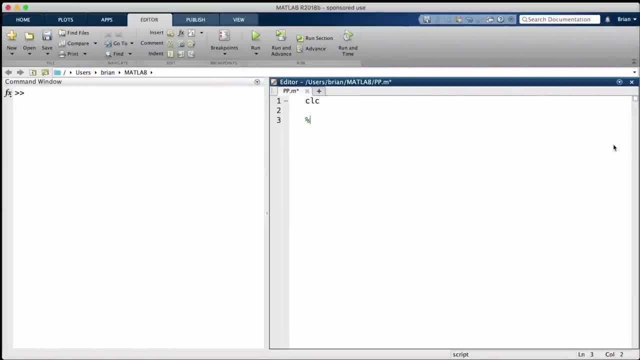 thing in MATLAB with pretty much a single command. I'll show you quickly how to use the place command in MATLAB by recreating the same system that we just did by hand. I'll define the four matrices and then create the open loop state space object. I can check the eigenvalues of the open loop A. 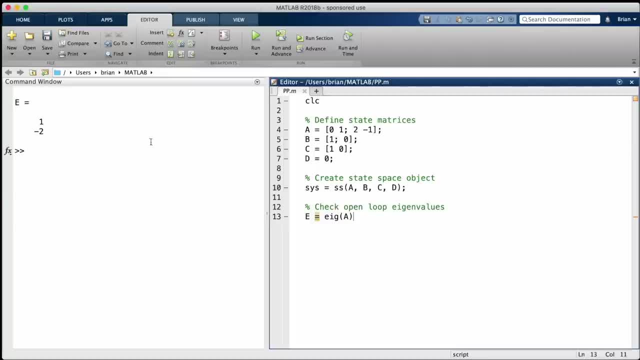 matrix just to show you that there is in fact that positive eigenvalue that causes the system to be unstable, And that's no good. So let's move the eigenvalues of the system to minus one, Minus two and minus one. Now, solving for the gain matrix using pole placement can be done with the: 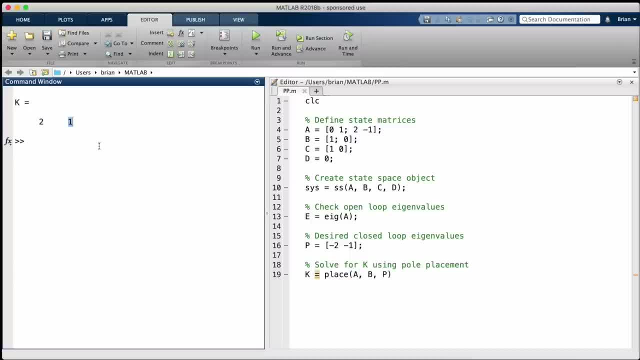 place command And we get gain values of two and one, just like we expected. Now the new closed loop A matrix is A minus BK And just to double check, this is what ACL looks like and it does have eigenvalues at minus one and minus two. Okay, I'll create the closed loop system object and now we can compare. 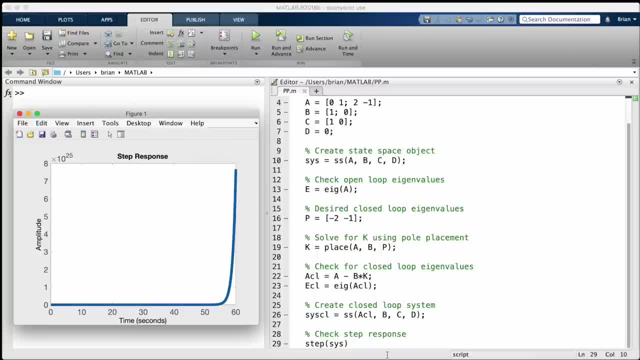 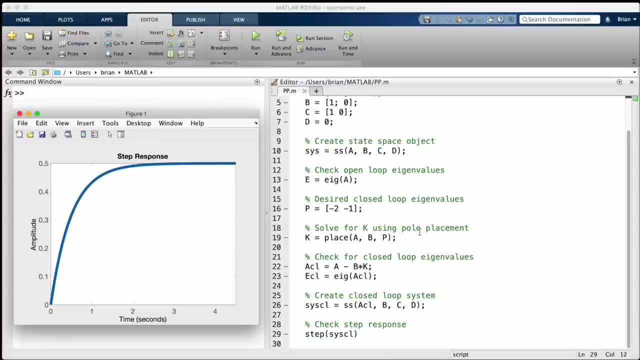 the step responses for both. The step response of the open loop system is predictably unstable, And the step response of the closed loop system looks much better. However, it's not perfect. Rather than rising to one, like we would expect, the steady state output is only 0.5.. 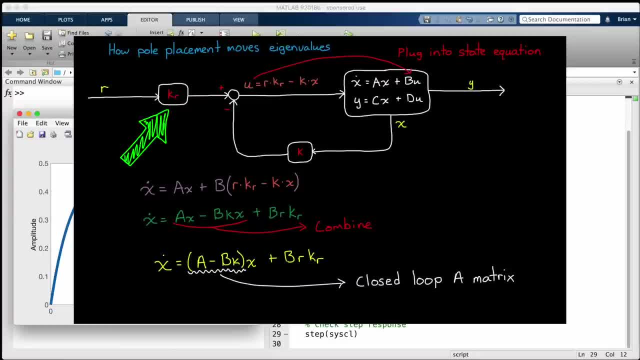 And this is finally where the scaling term comes in. on the reference, So far we've only been concerned with stability and have paid little attention to steady state performance. But even addressing this is pretty straightforward. If the response of the input is only half of what you would expect, why not just double the input? 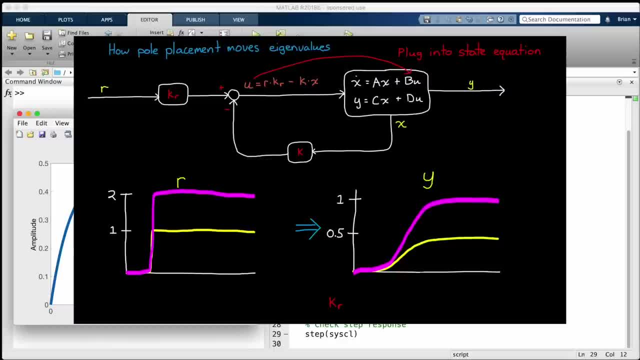 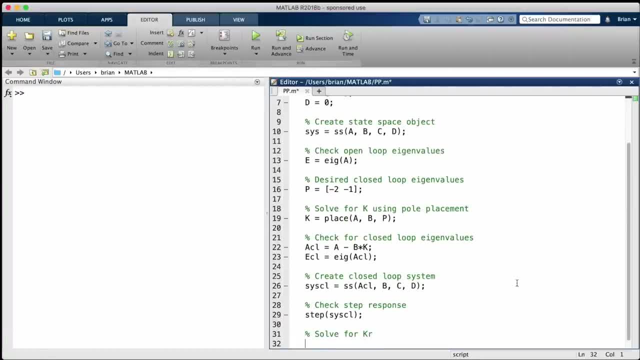 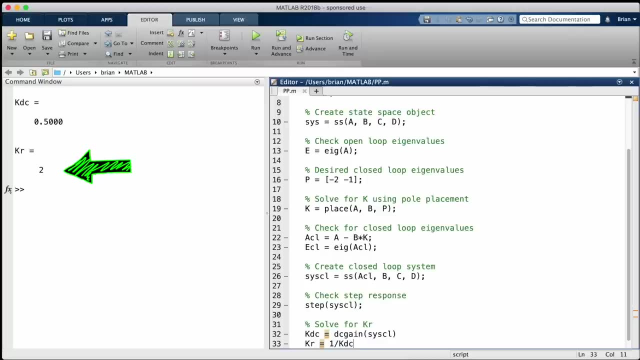 And that's pretty much what we do. Well, we're not just doubling it, We scale the input by the inverse of the steady state value. In Matlab, we can do this by inverting the DC gain of the system. You can see that the DC gain is 0.5, and so the inverse is 2.. Now we can rebuild. 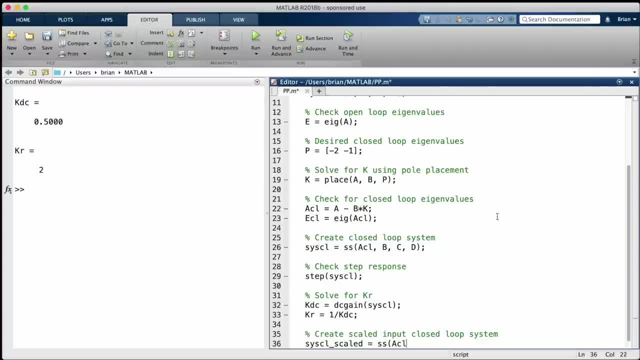 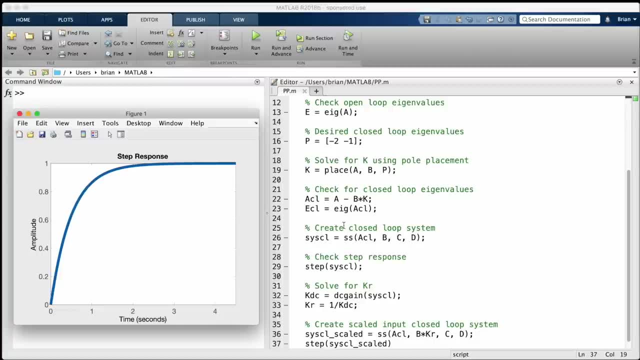 our closed loop system by scaling the input by K are or by two and checking the step response. And no surprise, its steady state value is one. And that's pretty much what there is to basic pole placement. We feedback every state variable. 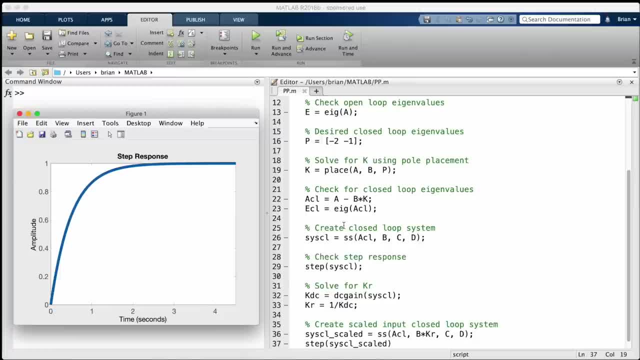 and multiply them by a gain matrix in such a way that the closed loop eigenvalues are what we want and then we scale the input to make the steady state response what we want. Of course there's more to pole placement than what I could cover in this 12 minute video. 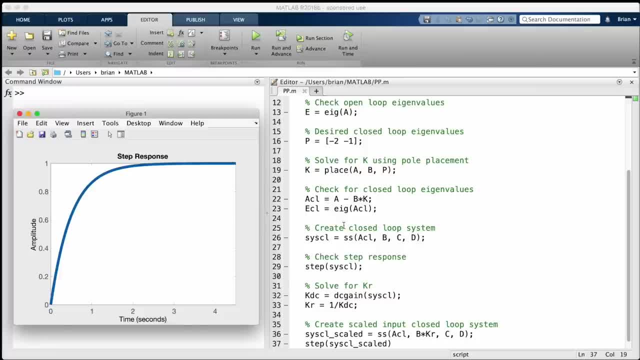 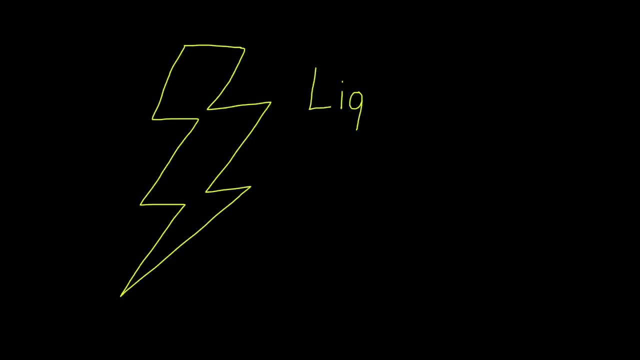 And I don't want to drag this on too long, but I also don't want to leave this video without addressing a few more interesting things for you to consider. So, in the interest of time, let's blast through these final thoughts lightning round style. Are you ready? Let's go. 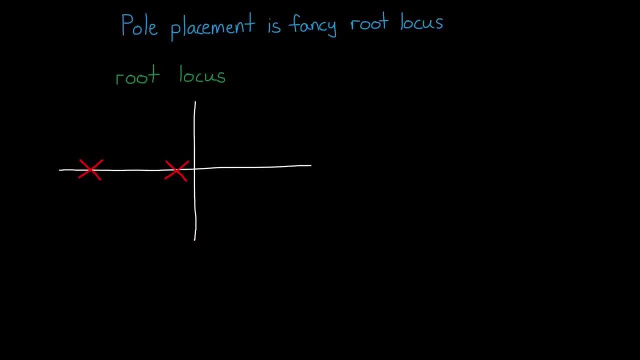 Pole placement is like fancy root locus. With root locus you have one gain that you can adjust. that can only move the poles along the locus lines. But with pole placement we have a gain- matrix- that gives us the ability to move the poles anywhere in the complex plane. 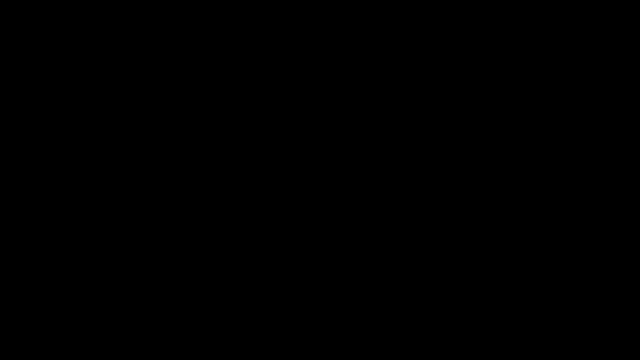 and we can move the poles anywhere in the complex plane, Not just along single dimensional lines. A two state pole placement controller is very similar to a PD controller. With PD, you feed back the output and generate the derivative within the controller. With pole placement, you are feeding back the derivative as a state, but the results 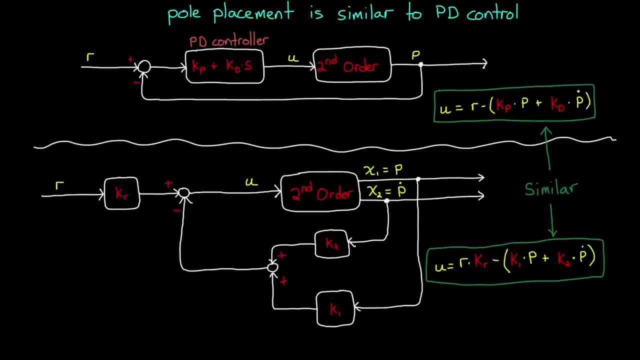 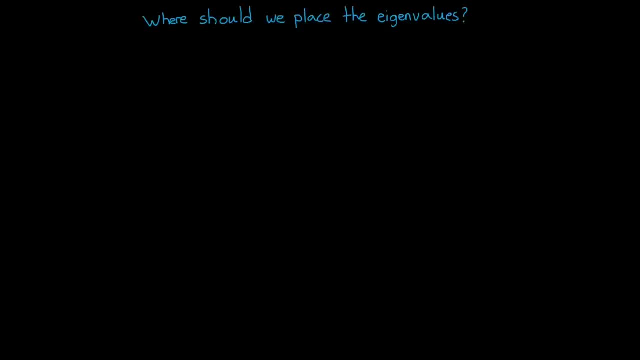 are essentially the same: Two gains, one for a state and one for its derivative. Okay, we can move eigenvalues around, but where should we place them? The answer to that is a much longer video, but here are some things to think about If you have a high order system. 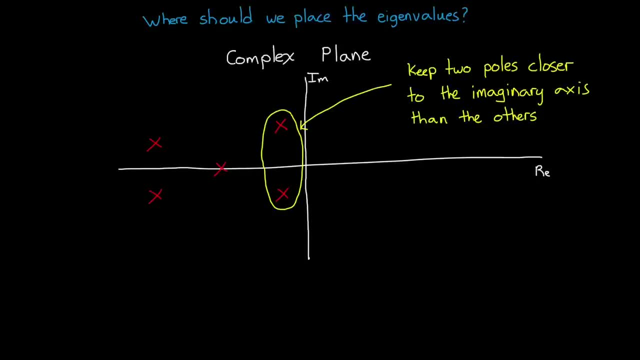 consider keeping two poles closer to the imaginary axis than the others, so that the system will behave like a common second order system. These are called dominant poles, since they are slower and tend to dominate the response of the system. Keep in mind that if you try to move a bunch of eigenvalues really far left in 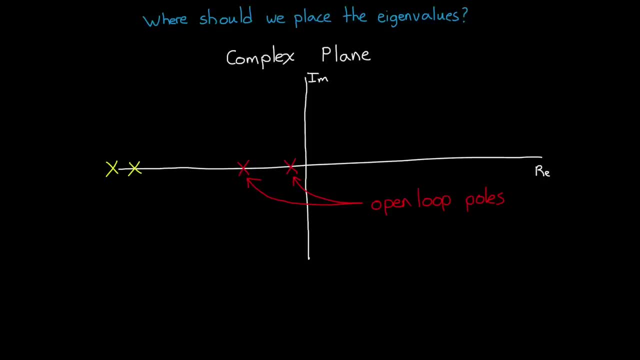 order to get a super fast response, you may find that you don't have the speed or authority in your actuators to generate the necessary response. This is because it takes more gain or a more actuator effort to move the eigenvalues further from their open loop starting. 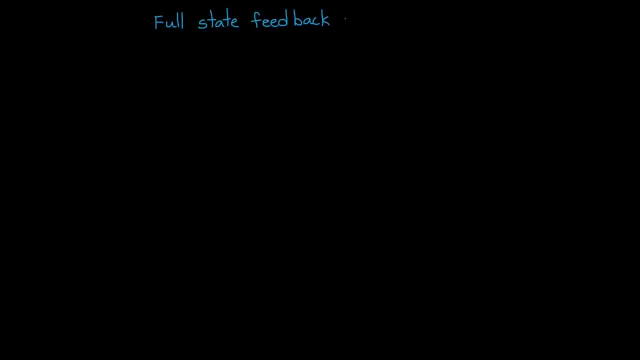 points. Full state feedback is a bit of a misnomer. You are feeding back every state in your mathematical model, but you don't and can't feed back every state in a real system. For just one example: at some level all mechanical hardware is flexible. 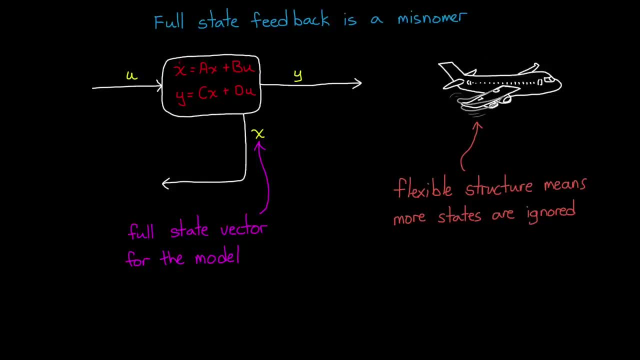 which means additional states, but you may choose to ignore those states in your model and develop your feedback controller assuming a rigid system. Now the important part is that you feed back all critical states to your design so that your controller will still work on the real 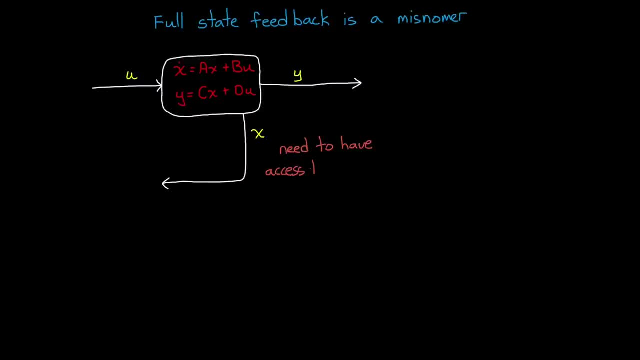 hardware. You have to have some kind of access to all of the critical states in order to feed them back. The output y might include every state, in which case you're all set. However, if this isn't the case, you will either need to add more sensors to your system to measure.